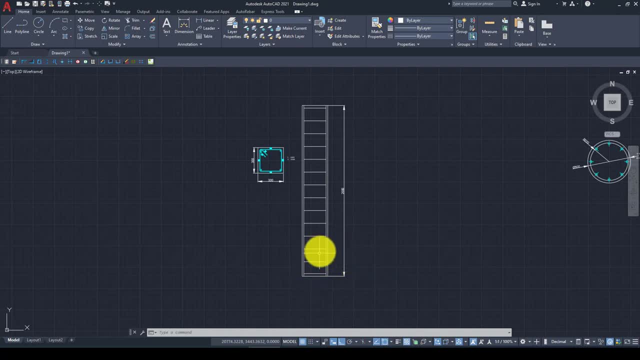 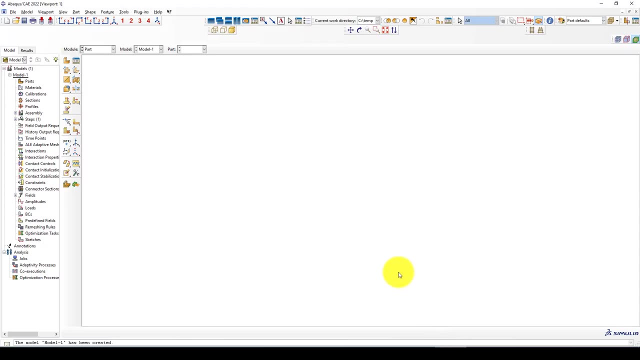 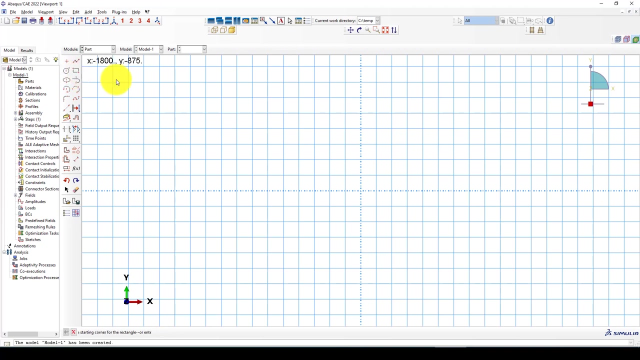 And then I will add some sort of shear failure on a concrete to see how the column behave. So we go to here and create a concrete. The concrete column is column. You can say 30 by 30, which is using a solid element, and I can select a rectangle and give minus 150 and minus 150 for the X and the Y direction. 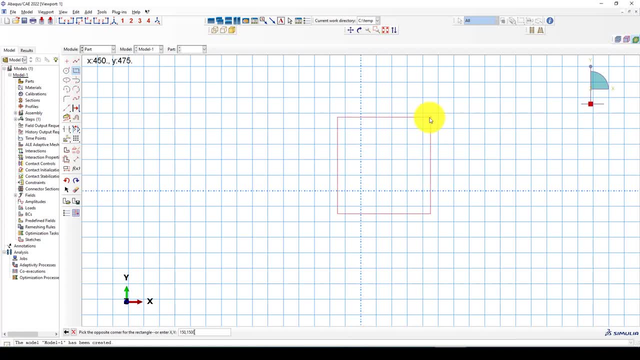 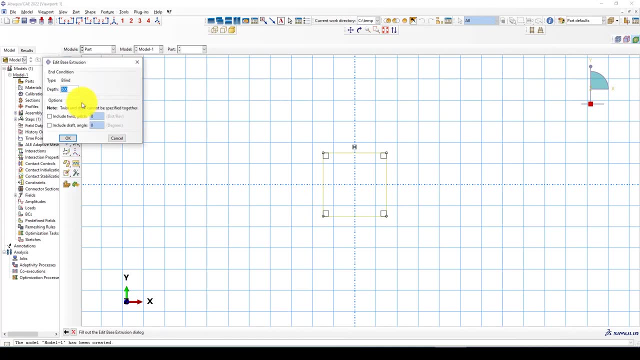 So now again 150 positive and 150 negative. So now again 150 positive and 150 negative. So now again 150 positive and 150 negative. So now again 150 positive and 150 positive. So the column is, the concrete section is created, and just let me give it in the depth or height, two meter. 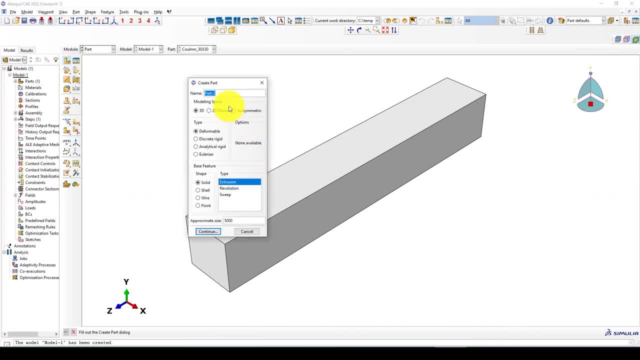 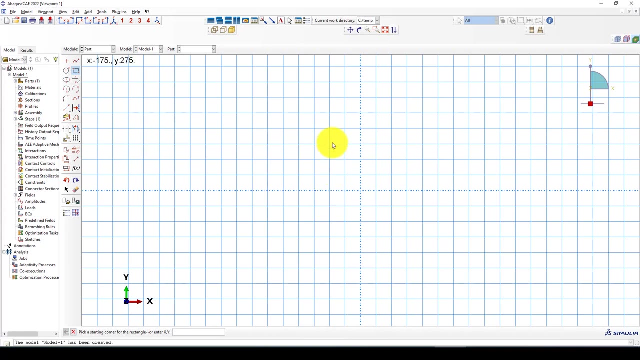 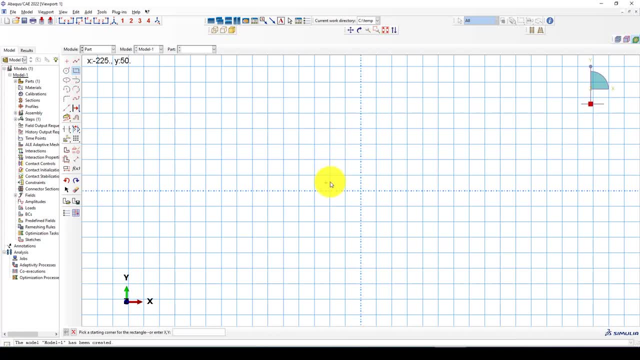 So the cover is a clear. cover is 20 millimeters. So the cover is a clear, cover is 20 millimeters. So which? reducing 21 side, 21 side, 20 top, 20 bottom. So for this now I can give 130 minus minus 130 and minus 130.. 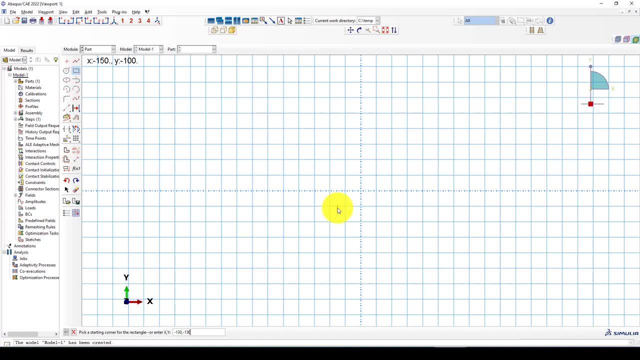 So for this now I can give 130, minus, minus, 130 and minus 130.. So, as a square shape, And now again, and who's it in 100? was it in 130?? And the strap is also, And the strap is also. 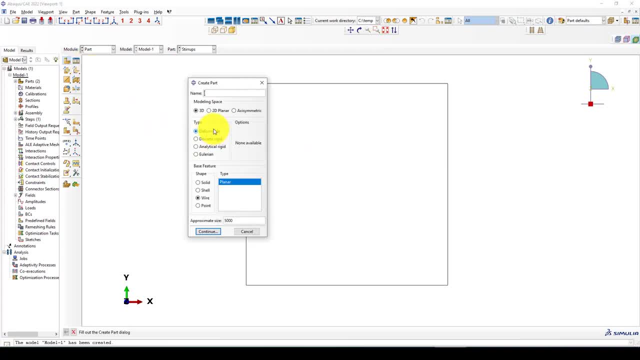 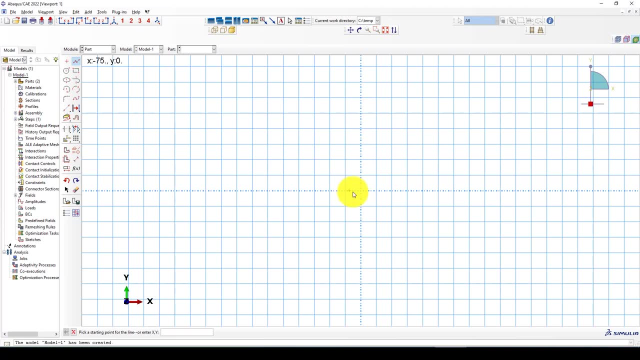 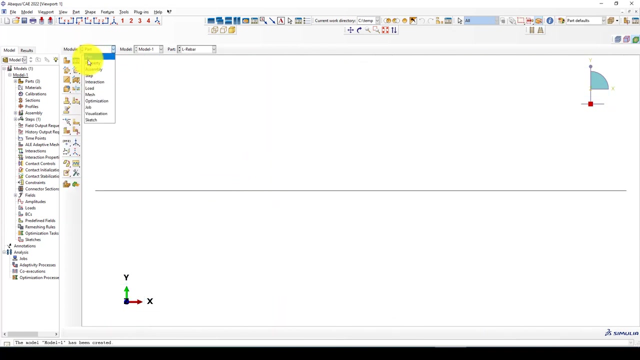 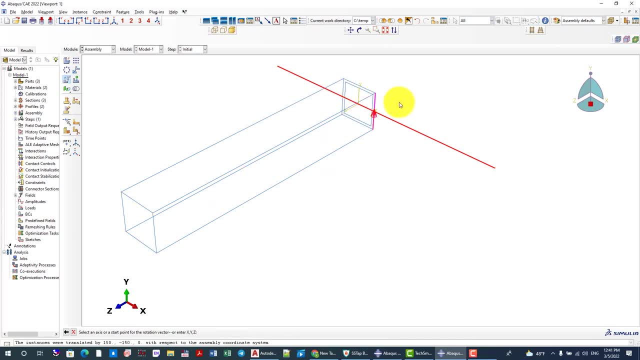 And now there's also completed, and the second part is defining material in the material we have. And now there's also completed, and the second part is defining material in the material we have. using this- and I want to take it at this point to this point and the next I want. 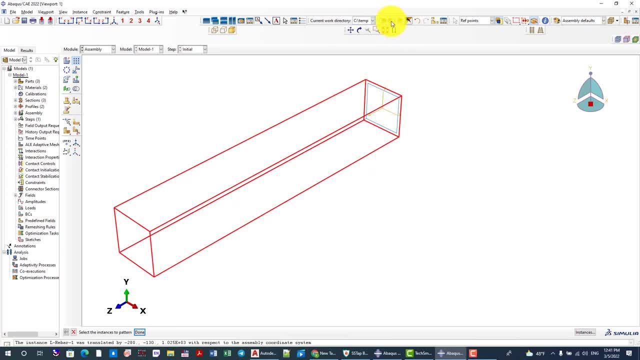 to populate that. so first select this one. I want to remove and select this one. populate other two corner 260 and this is also 260. now I want to make a little movement move of this reward to sometimes in during the interaction. it will not embed with the concrete. so taking 0.0 and in the Z direction, want 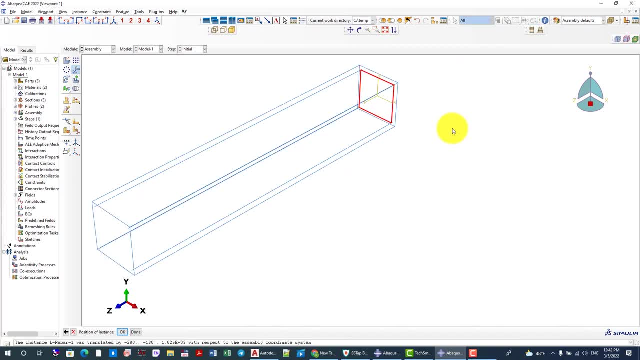 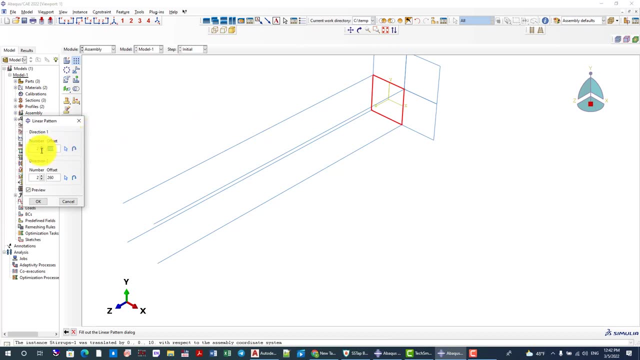 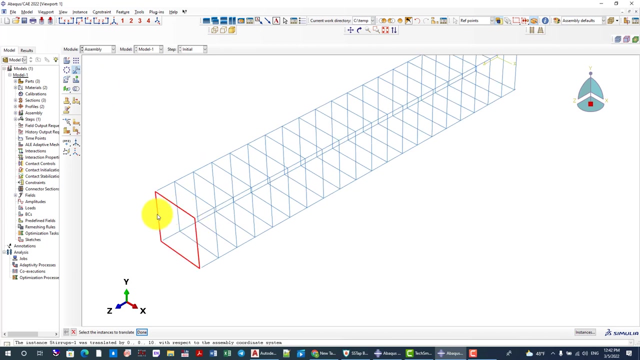 to take it 10, 10, 10, 10 millimeter. now it's okay. now I want to go to the select. this one I want to give 100. so this direction and front, I'm going to populate it to end of the structure, okay. and the last one is a little front in my 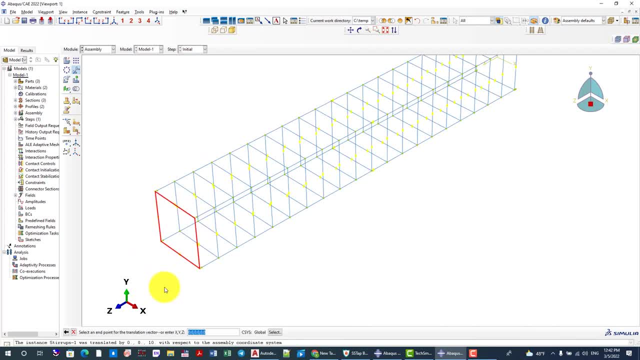 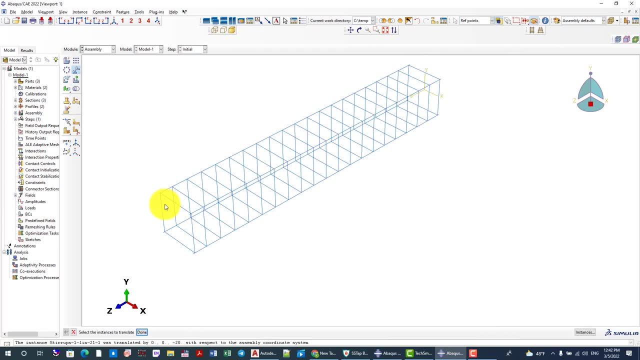 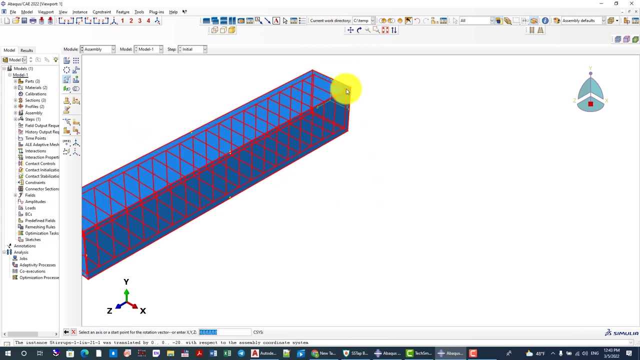 going to select 0: 0 and the second point is going to 0: 0 minus 20. so it's correct now. so we finished and select all and rotate, make it in a y-x plan, and one more thing is to bring it to origin. 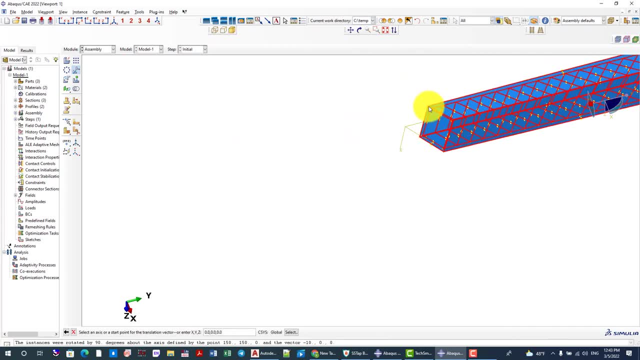 and this point to 0: 0 and now it's fixed and we're going to define a step. so this is okay. okay, and go to step in this part. just, I want to consider a standard solver or static analysis, and the second part, which is the evolution of the, the, the. 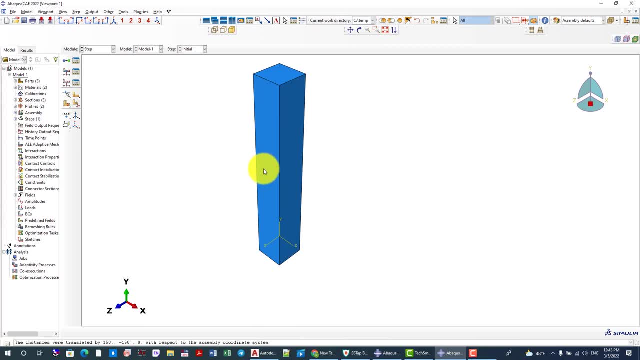 overlap in the field 다른 Robot. in the next step we're going to define the aberration of the loss. so this will definitely happen. it's a decrease here, very. there will remain the be a کار بي Esc and, Rob, that is now be a volume instead of constant, of significant termかな. 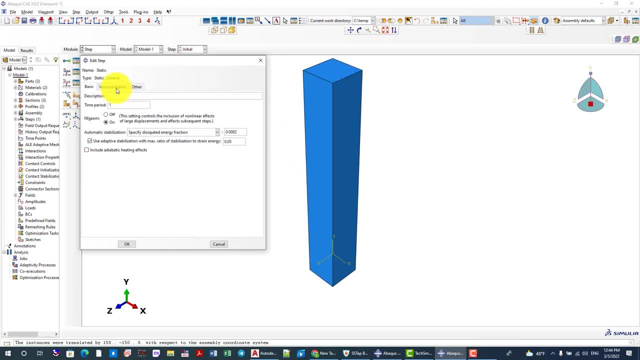 yes, okay, energy fraction between the concrete and rebar and time period is, let's suppose, 10 second and i'm going to a very large number. so during the analysis there is no lack of increment. so, going to 0.0105, a small one, and 1 e minus 15, very minimum increment. 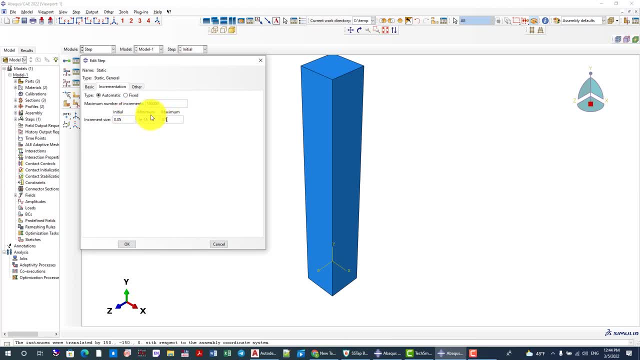 and this is 0.1. so we will slowly apply the displacement in the top of the structure and then see the structure response or draw the curve of the force displacement. this is okay and we can. before that, i'm going to draw some some point, center point. i'm going to take one here. 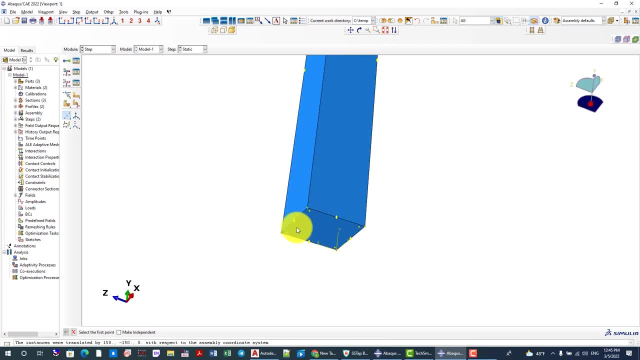 this is one center point of the column. uh, also one center point here. in case the concrete is not eccentricity, then you can apply the eccentricity percentage, uh, shifting this by uh, some lateral difference. let's suppose you have this option. you can take this point and define a little other side. 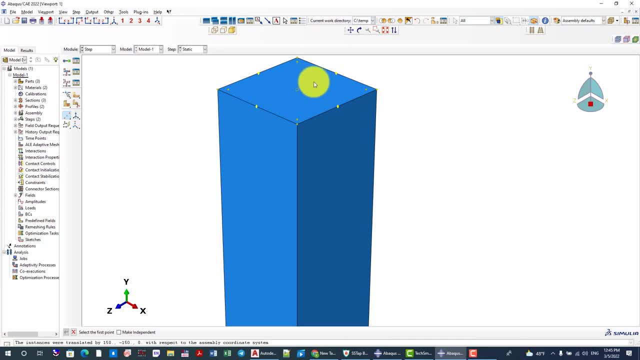 so the loading will be: uh, unconcentrated, equal to concentrated. so the concentrated load is change to unconcentrated load so that you will give different response curve. so now it's a concentration legally curve, uh concentrically loading step, which is seems that structure is located in the. the column is located in the center of the building. 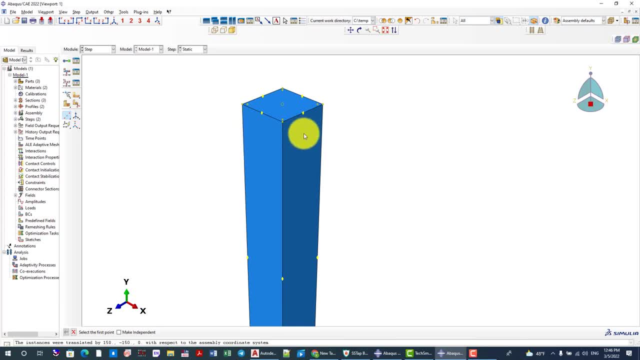 in case you have in the edges, on the, in the corner, so that you have to consider that it's a concentricity and that the concentricity can be a topic for discussion and for analysis of such kind of column. now I want to create a reference point in that. 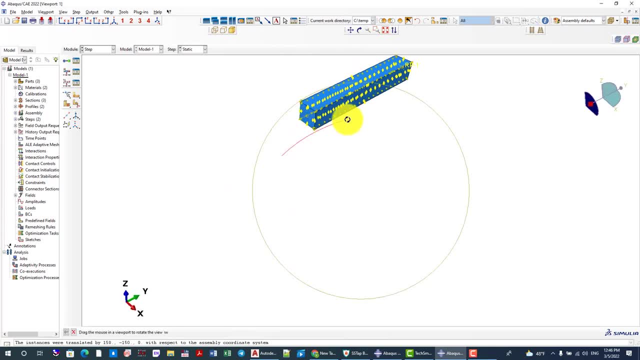 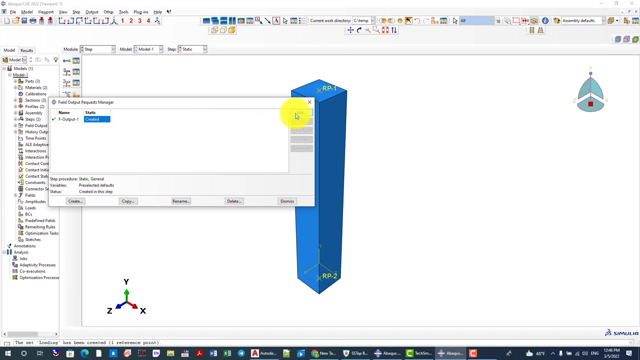 area. so one reference point for binary condition, one reference point for looting, and I want to create a mood called looting point, in that I different. point one is the loading point, and what I want to do is just: first of all, let me go to define some other parameters, such as their concrete 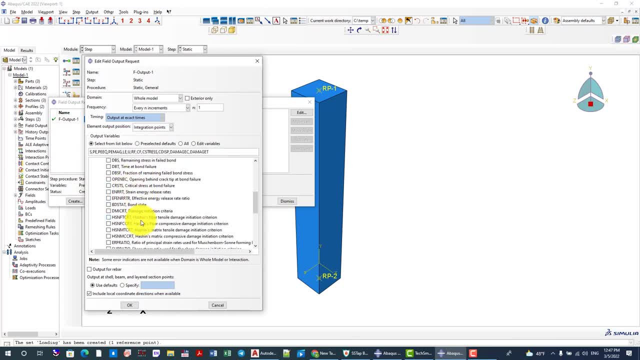 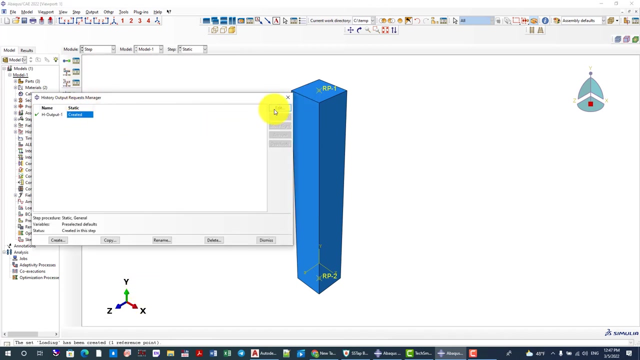 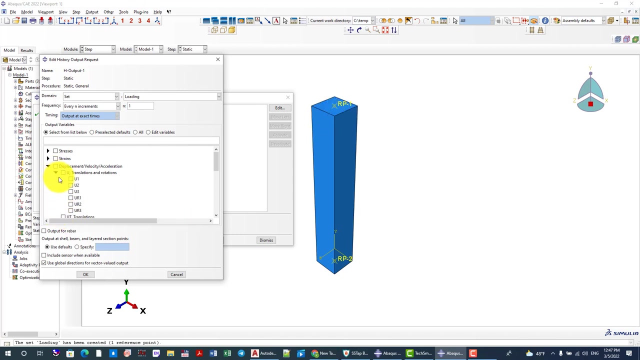 damage and also scholar degradation, scholars technique addition, this one, and also we can go to the state field variable and using this command and output is: every increment is one. okay, now, No, here I want to get, just using that sit loading and I want to get the vertical load and also vertical displacement of that point going to you. 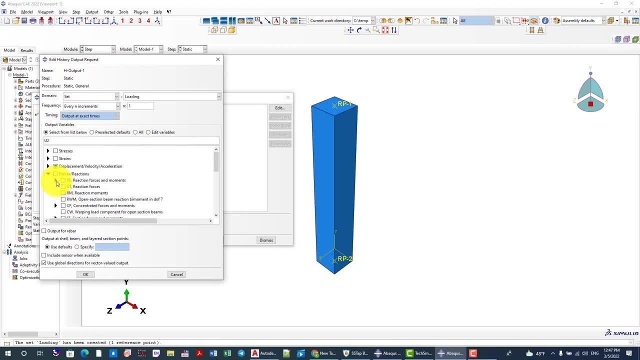 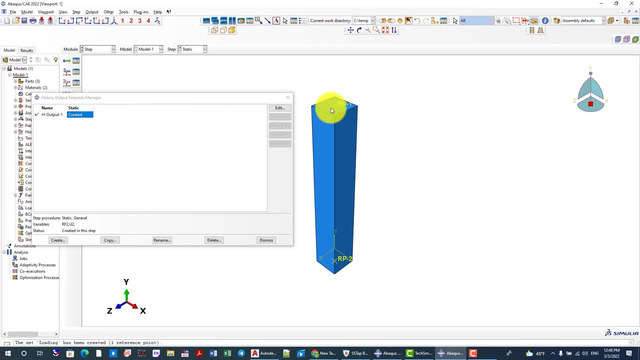 too, and re f2. so first we will apply the displacement- actually we, we usually use a sort of device- and then loader support and pushing them down, and then we will. there is some reaction force, so that reaction force in the finite element is equal from the bottom to here. so and the next step? instead of that pushing if displacement, 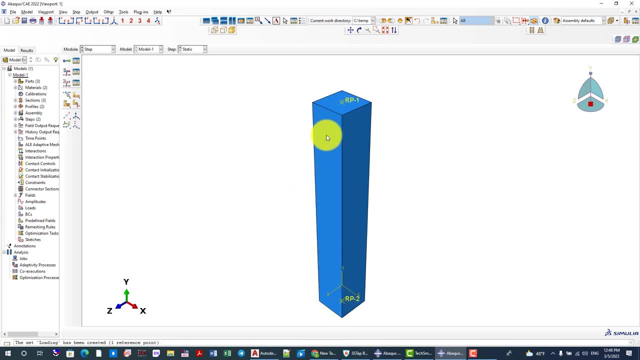 we will use the load which we got from these analysis and then we will see the response of that structure. well, we show it's quite simple, which is that it will apply with a different kind of hexagonal system, so that we will use the same thing. so 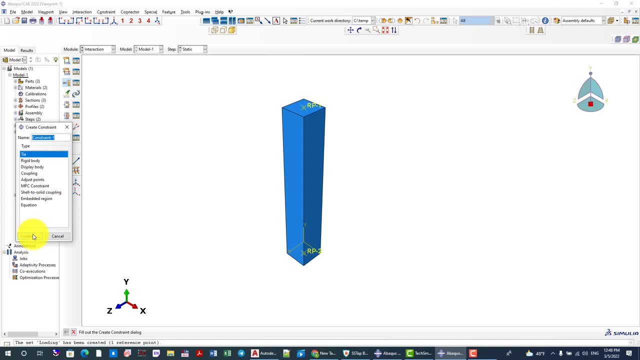 we can jump to the point where we need and then we can close it and we can match it, so we can expand it in that way. and if I have no interaction, any interaction, just, we have two interaction. we can use coupling or tine- but that means we want to tie these node to the entire surface- or coupling. so both are okay, lets make it coupling. so the coupling one is they. at this point I can select that geometry here and then go to node, region or 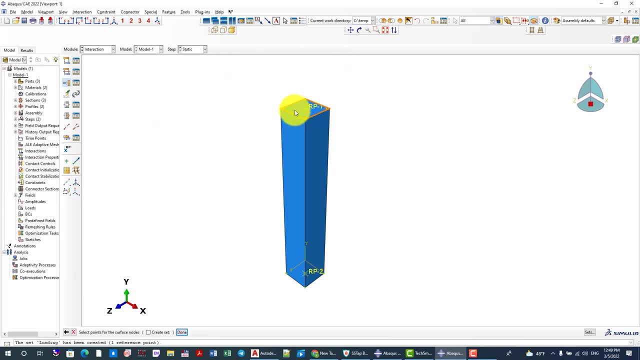 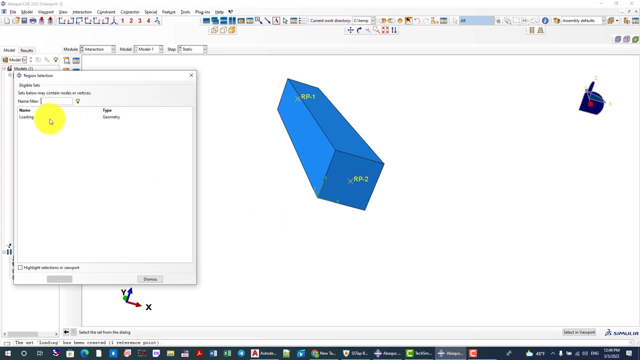 in that way, so I can select that geometry and then go to node region, or, and then go to node region or displacement. so here is, and I can see so that, so that also representing the load will distribute equally to entire elements, entire surface. now again I can go to second here. this time I want: 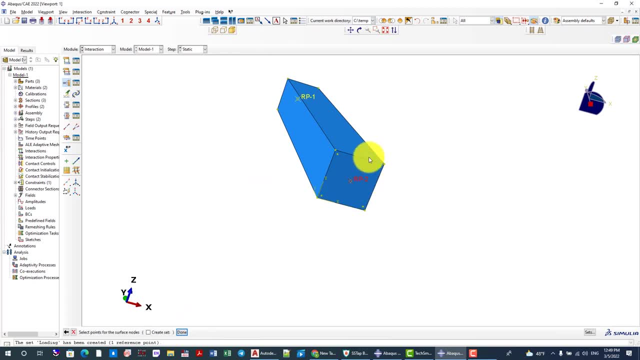 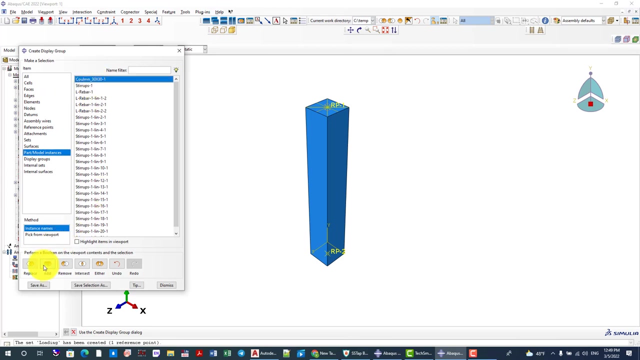 to take this point is control point and note region, yeah, which I created both. and the last interaction is in bed, the embedded region, which is interaction between concrete and rebar. I'm going to pause and I can going to column, so remove it and I can select all those. and I can select all those and I can remove it, and I can select all those and I can remove it, and I can select all those and I can remove it and I can remove it, and I can remove it and I can use still and I can go to. 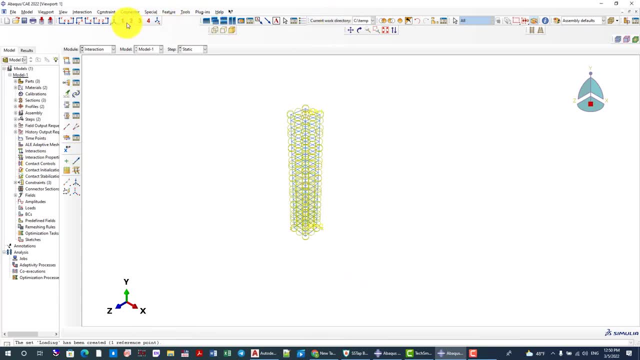 it and I can remove it and I can use still and I can go to it and I can remove it and I can use still and I can go to all models. and now here is and I can show all models. and now here is and I can show. 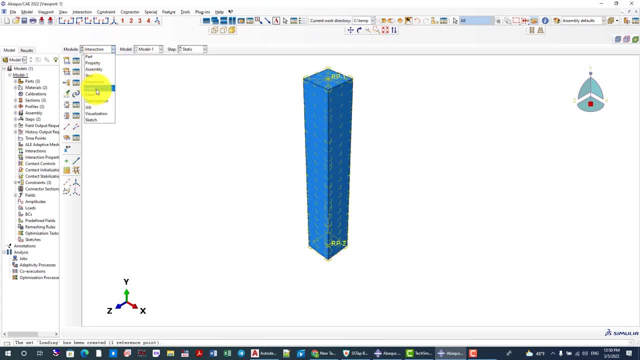 all models. and now here is, and I can show everything: now injection is finished, we, everything. now injection is finished, we everything. now injection is finished. we go to the loading, and so we both use an go to the loading, and so we both use an go to the loading, and so we both use an initial, first called fixed, base, fixed. 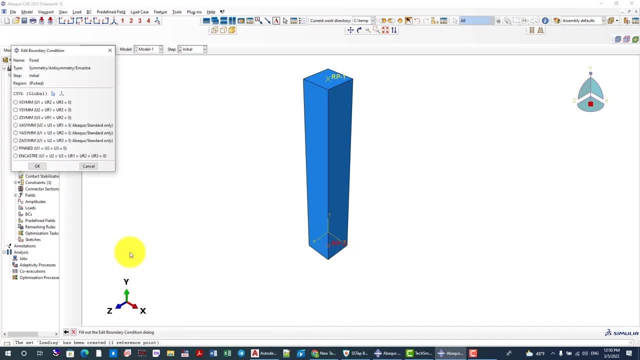 initial first called fixed base: fixed initial. first called fixed base: fixed base and I'm going to select this point base and I'm going to select this point base and I'm going to select this point as a fixed in caster and the as a fixed in caster and the. 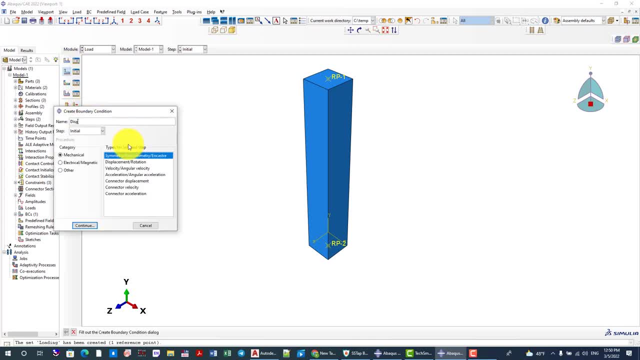 as a fixed in caster and the thicken. is that top call displacement and this is thicken. is that top call displacement? and this is thicken? is that top call displacement? and this is in a static, so I'm going to in a static, so I'm going to. 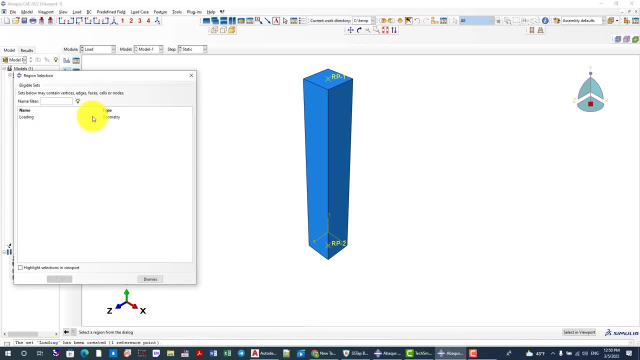 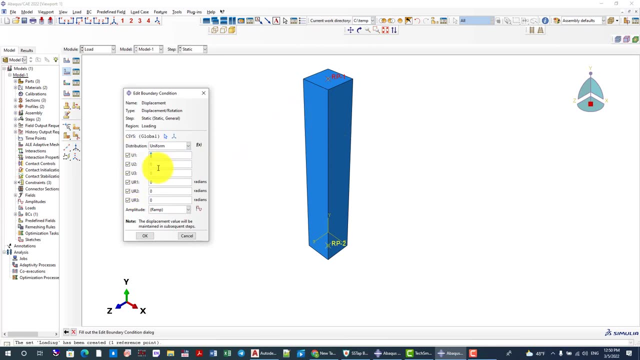 in a static. so I'm going to select displacement and selecting that point, select displacement and selecting that point. select displacement and selecting that point, which already defined here now I, which already defined here now. I, which already defined here now, I want to restrain all other direction except. 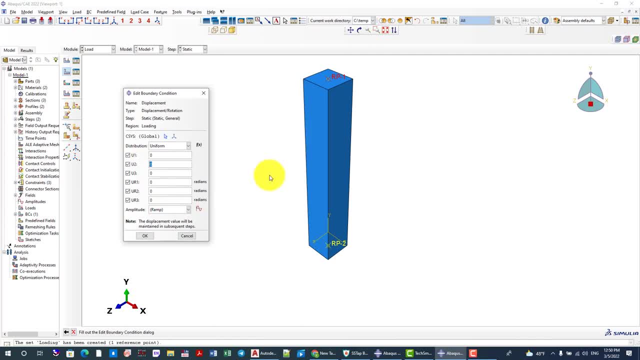 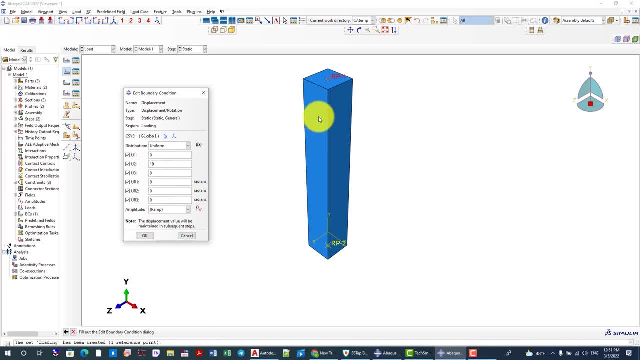 is going to push this to one centimeter, so is going to push this to one centimeter. so during one centimeter. so concrete is a during one centimeter. so concrete is a during one centimeter. so concrete is a brittle material and it will start to 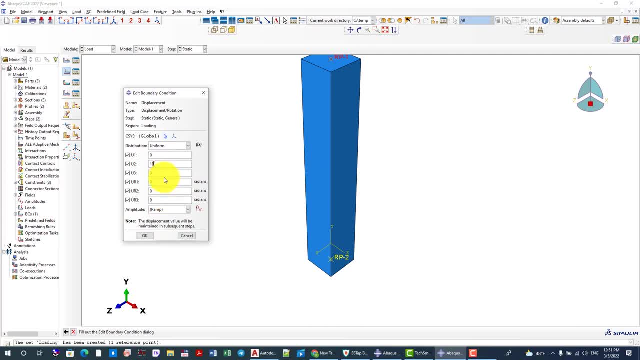 brittle material and it will start to brittle material and it will start to crack and crash. or I can give 20 milli crack and crash, or I can give 20 milli crack and crash, or I can give 20 milli. to see more information. this is that. 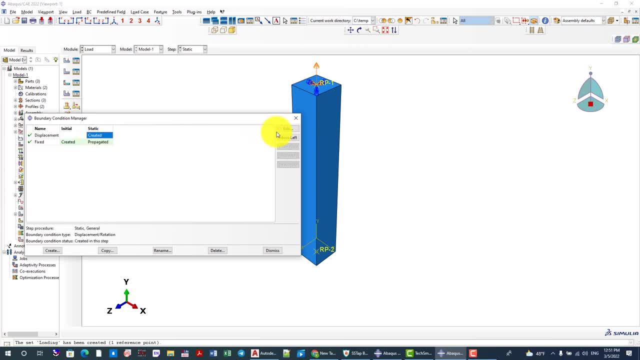 to see more information. this is that: to see more information. this is that should be in a negative direction. is should be in a negative direction. is should be in a negative direction. is PM minus 20 to get down. PM minus 20 to get down. PM minus 20 to get down. now the loading is finished, so the last. 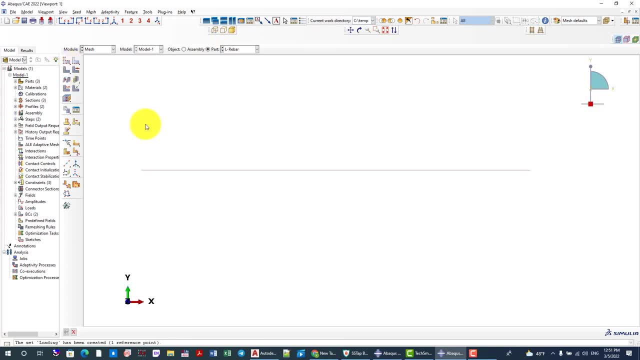 now the loading is finished. so the last: now the loading is finished. so the last thing is mission: we go to part. and here thing is mission we go to part and here thing is mission, we go to part and here is mission, giving 100 and stirrups and 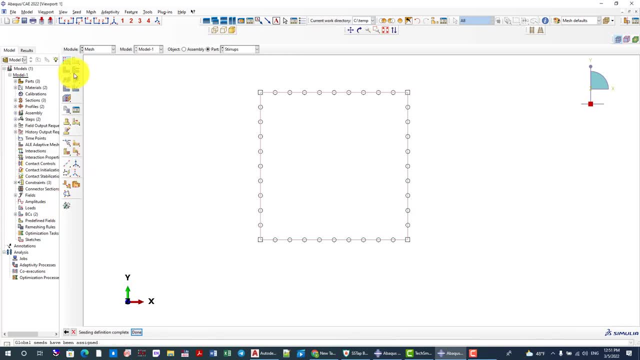 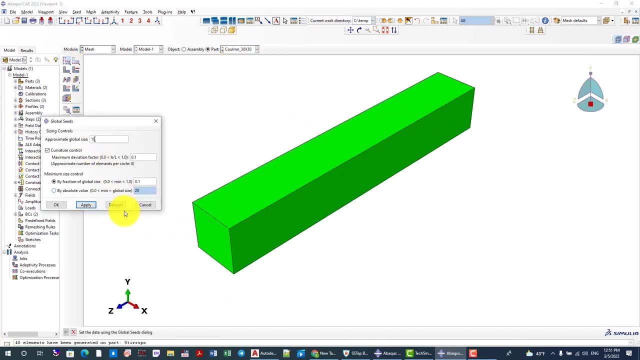 is mission giving 100 and stirrups and is mission giving 100 and stirrups and skip 25 and concrete and the concrete skip 25 and concrete and the concrete skip 25 and concrete and the concrete is going to 100, is going to 100 and 100. 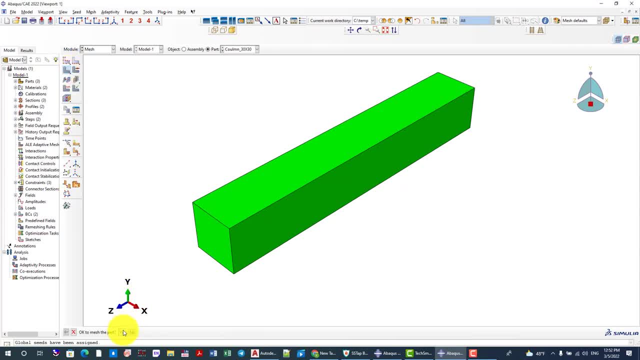 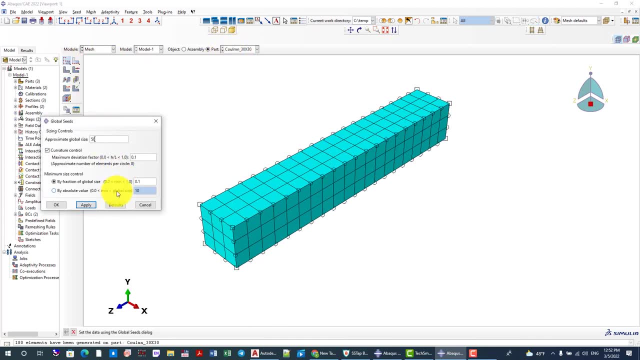 is going to 100 and 100. so this is very small course mesh and I so this is very small course mesh and I so this is very small course mesh and I want to make this one- 250, it's a little- want to make this one- 250, it's a little. 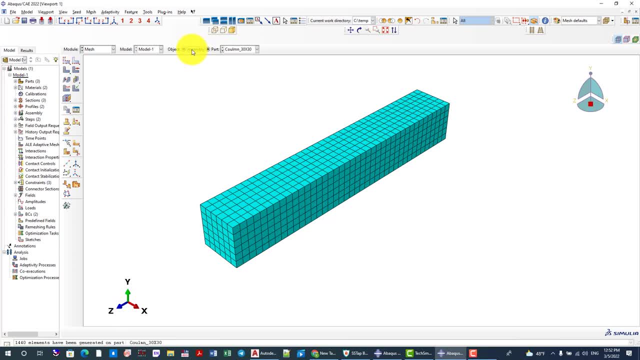 want to make this one 250. it's a little bit fine mesh. now it's better, so we can bit fine mesh. now it's better, so we can bit fine mesh. now it's better, so we can go to the finished with the job and go to the finished with the job and 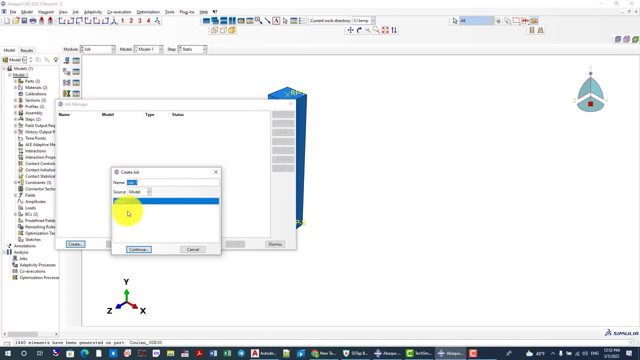 go to the finished with the job and this time we can create. this time we can create model 1- it's called model 1- and submit it. it's called. the following posts have been element without any section, so the concrete is: forget to mesh and assign a. 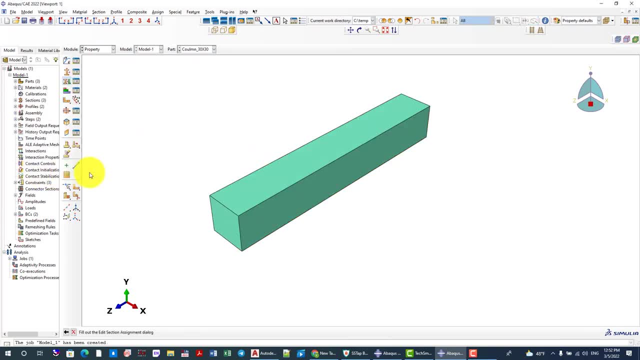 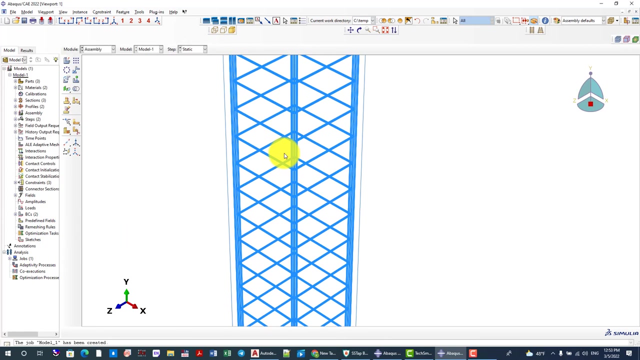 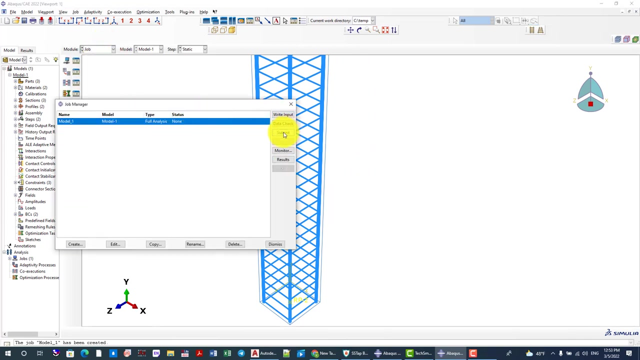 section. so here is the section concrete. another is okay. one more thing. I want to show you and the family that going to here, going to rebar and display option, and I want to see that this is the reinforcement rendering. so go to job. and now I want to submit again. 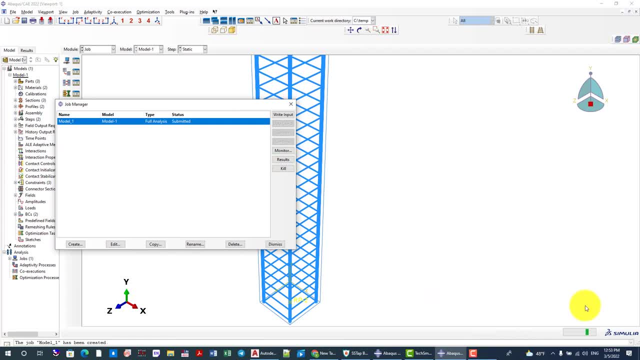 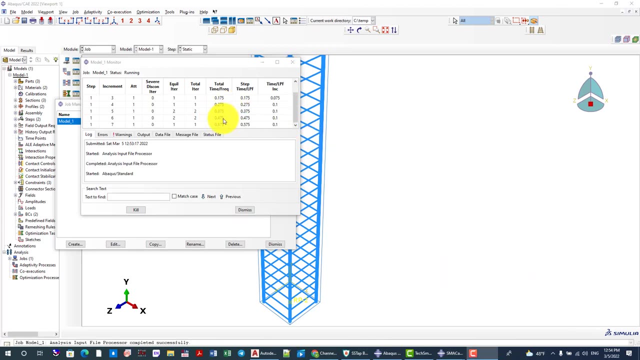 Joe is submitted and I want to consider the monitoring to see if there is any error to fix. and now it's starting 0.7 and it's it's quite cool and almost reached to one second. so I need to finish 10 second so then we can see the. 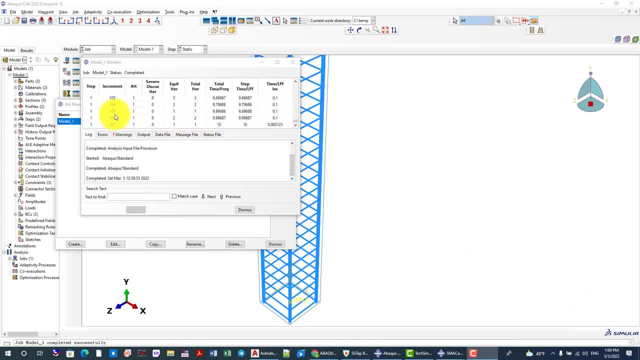 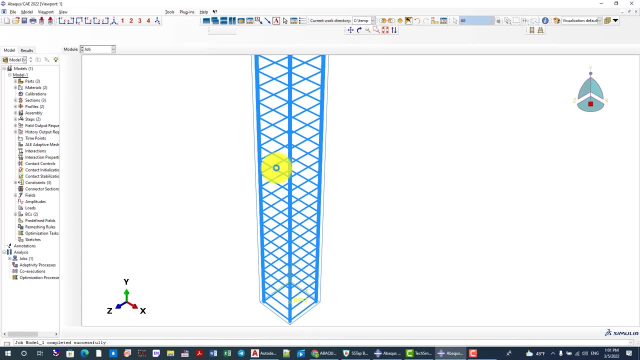 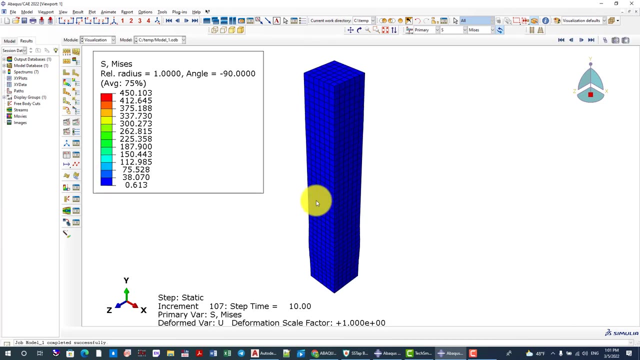 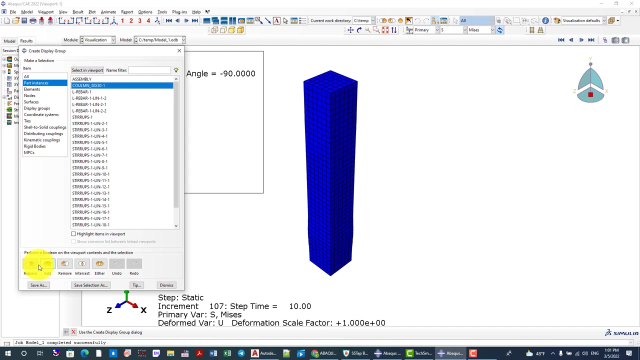 result. now the analysis completed and it took about 107 step, equipment steps. I'm going to call result. this is the result and this is first one miss: stress which is reached a yellow point, and I'm going to here and just go to part and replace and this is the concrete column stress, but it didn't reach to the 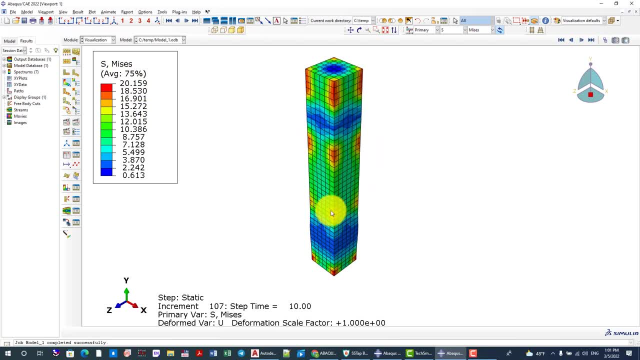 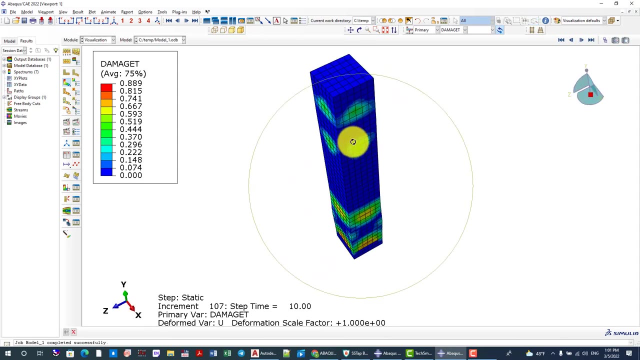 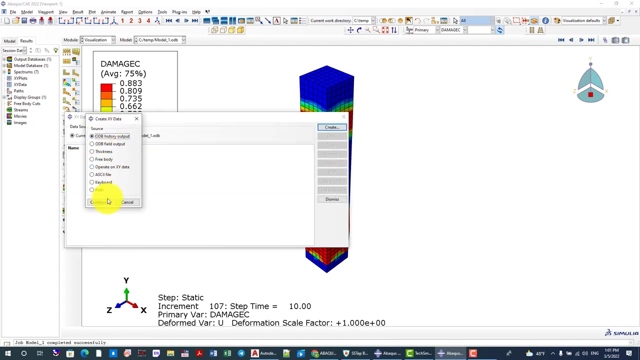 comparison field because concrete compressive strength is very high, it can resist a very large compressive load. if I go to the concrete tension damage, so this partially this area, this area and some other area is damaged also in the comparison. damage also occurred in bottom and top. now I want to see the response curve went to the OTP output. 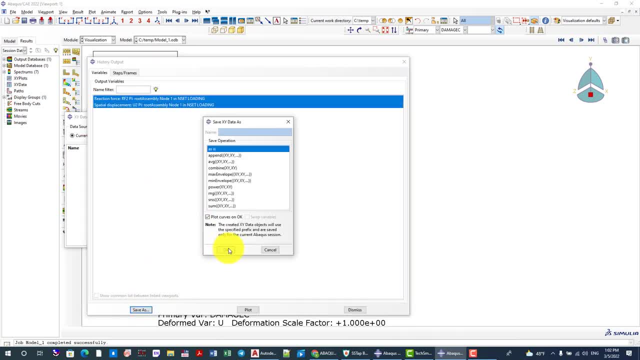 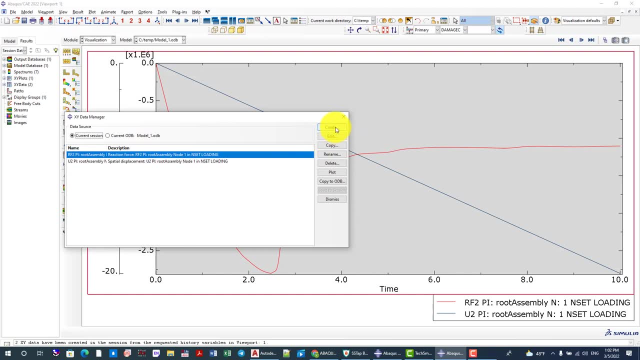 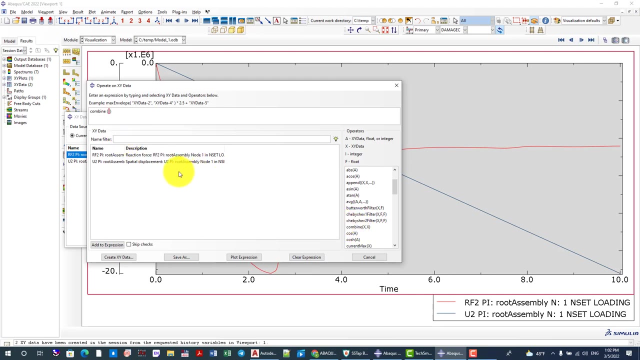 and we giving these two curve, and here is the curve, and here is the curve, and I want to create a FTP curve. now here is combined and times minus one because it's in a negative direction, and for both minus one times the reaction. we're going to save it to FD. 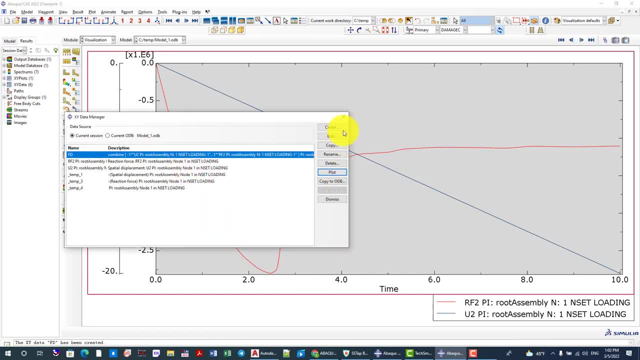 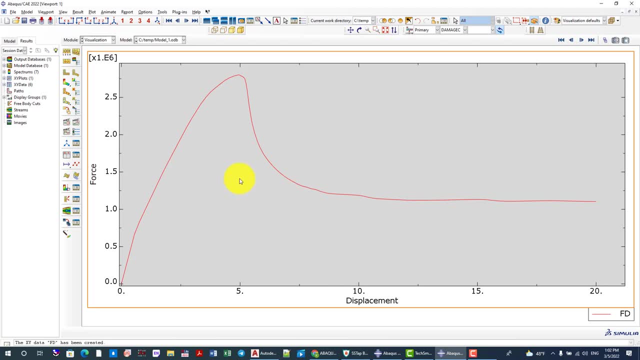 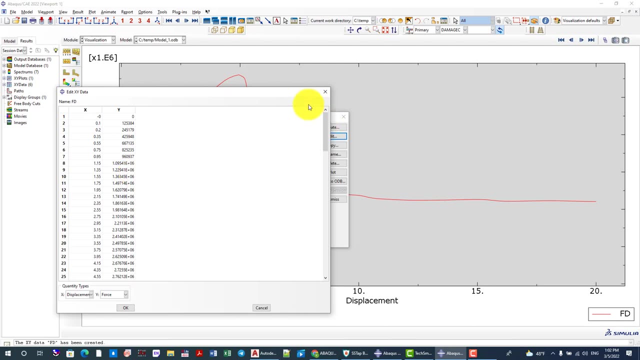 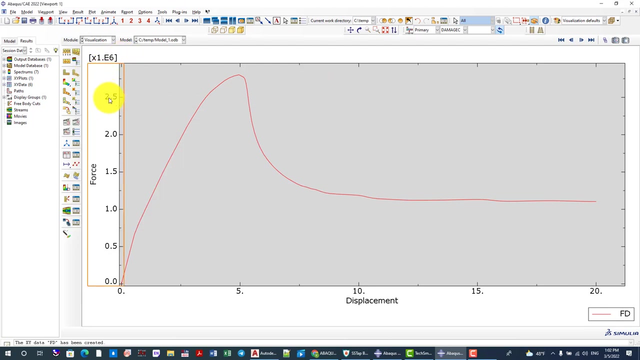 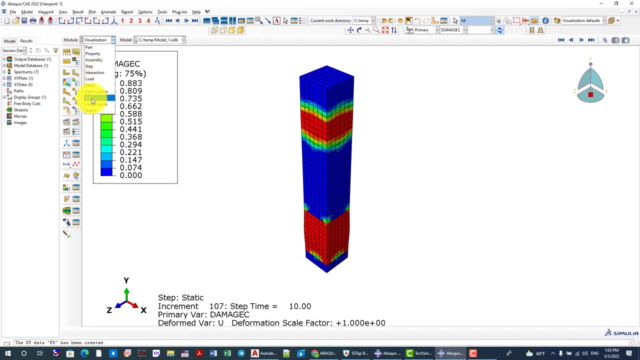 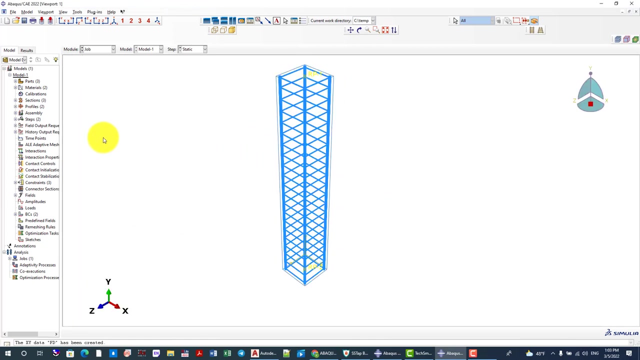 forces placement. going to plot and here is this is that component behavior and we can go to see the maximum displacement. so this is new to the IV in b. two I'm and the correct if aquesta am next tutorial. I want to get this data, use this data and this is the data and 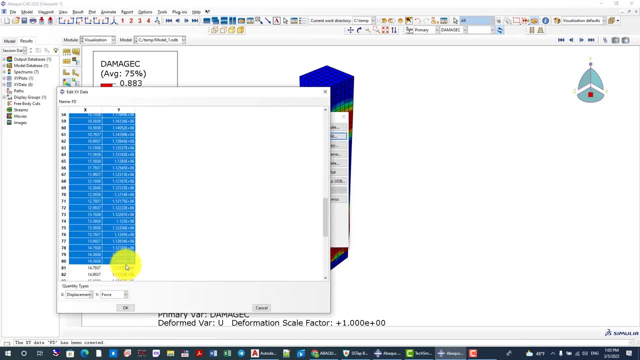 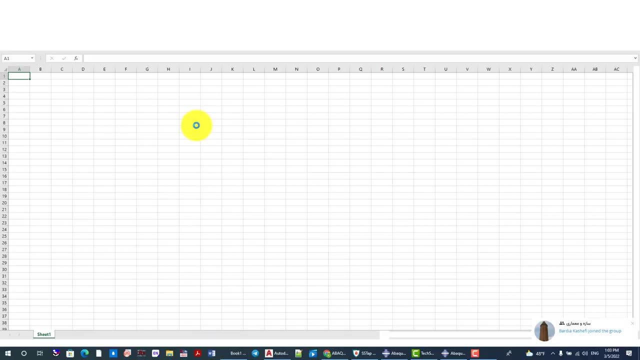 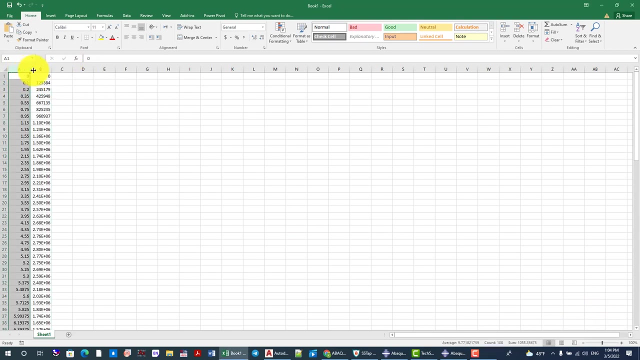 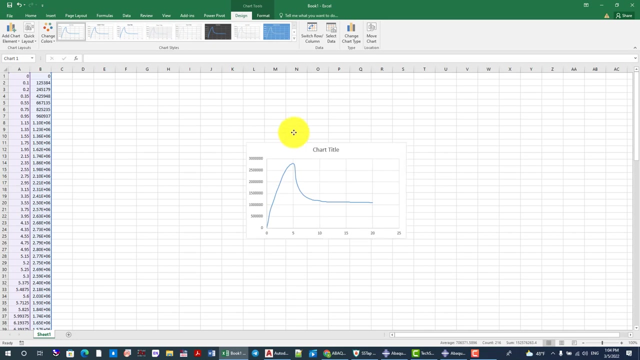 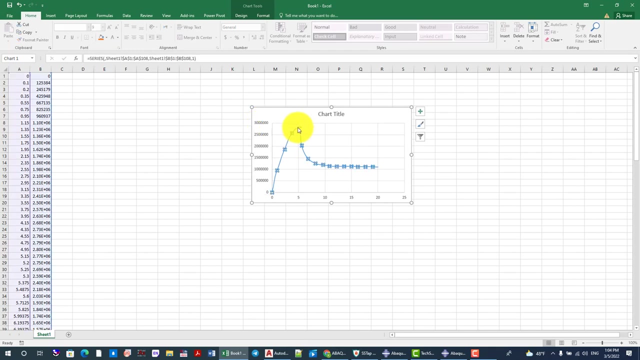 I'm going to export it. so the maximum. okay, I can go to copy to excel sheet and paste it to excel sheet and I can again click here, insert a graph force. so here is and that compressive string. now I want to see that the maximum of this. 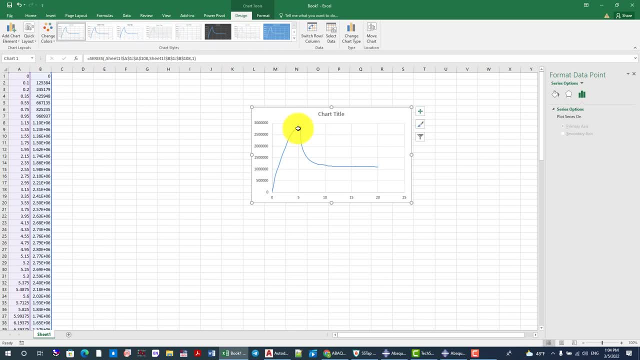 point is here. this is the total capacity of right here and here, and this is the total capacity of this point now going to or ultimate bearing. so it is about 4.9 and two thousand two thousand three kilonewton, two thousand eight hundred two kilonewtons. so four point nine five millimeter.